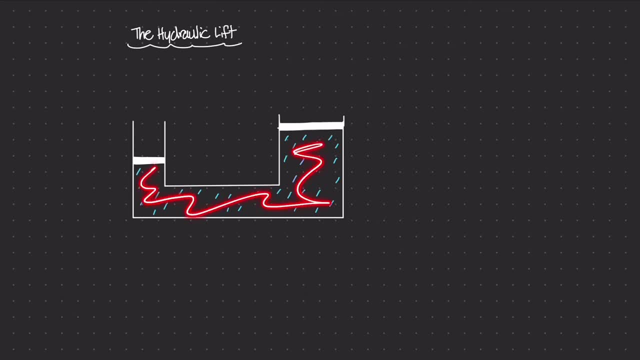 And inside of the system we have this liquid that has a constant mass density. So this fluid here has a row, this mass density, and this mass density is constant, And that's what we're going to talk about in this video, And that means that the fluid contained inside of this system is incompressible. So the concept of hydraulics is when we can use pressurized systems to do work and the underlying factor that's powering that work is Pascal's principle. 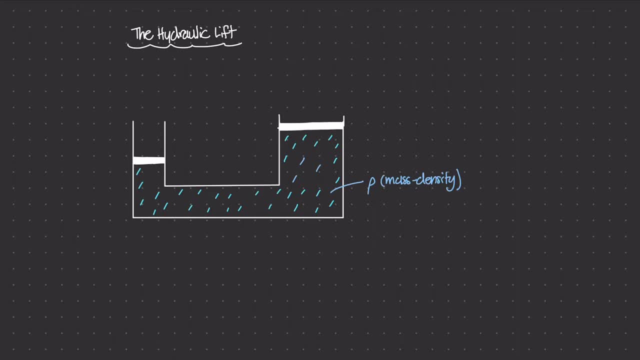 So let's say we had a car and the car was sitting here on piston two. So this is going to be my very poorly drawn cars. It has two windows. I'm sitting here on piston two, So I'm sitting inside and I'm happy. Now this car is obviously going to apply some sort of force going down on piston too. 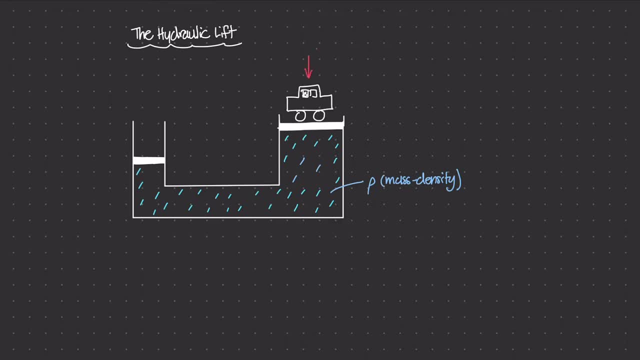 So I'm going to represent that by a vector here. This I'll just call force two, and that's being applied down into the liquid Now on the other side of the system. So on piston one, here we actually have a balancing force F1.. 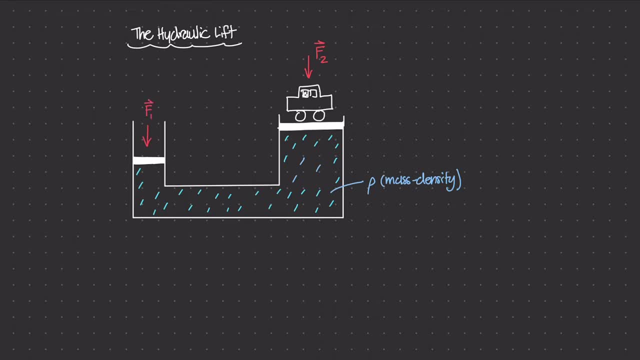 I'll just call F1. and this force is being applied down into the system and it's using this liquid, this hydraulic system, to counteract the force of this very big object, F2.. Now this works because, while the fluid is again, it's incompressible. but this 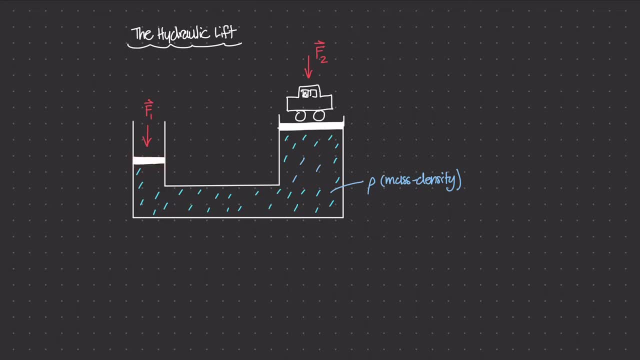 piston here on the left is smaller in area and we can use Pascal's principle to apply a very big force here on piston 2 to hold up the car. Now remember, Pascal's principle is: if you increase pressure at one point in the system, then that pressure increases, transmitted through all parts. 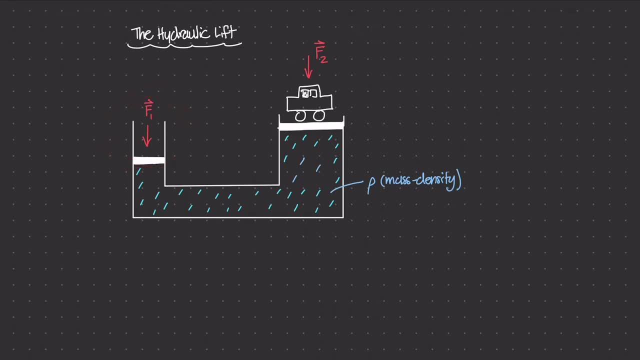 of the system. So on piston 1 we have this F1 force here that is applying some sort of pressure here at this point and because this is a hydraulic system and this state is in hydrostatic equilibrium with an incompressible fluid, then this pressure is going to be applied to the system. So if you increase pressure at one point in the 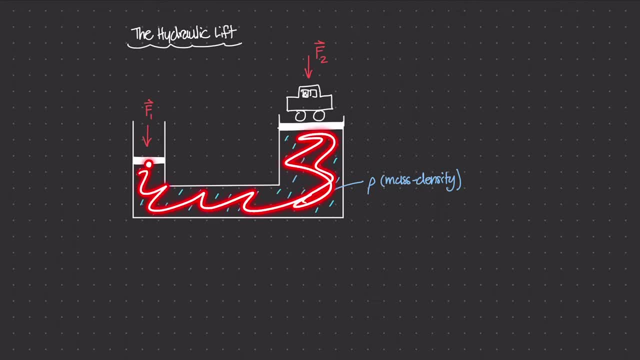 system, then that pressure is going to be transmitted to all parts of the fluid, including the fluid that's acting on piston 2.. So that pressure is going to apply against this big area for piston 2 and that's going to result in a much larger force than F1, but it's going to be a force that 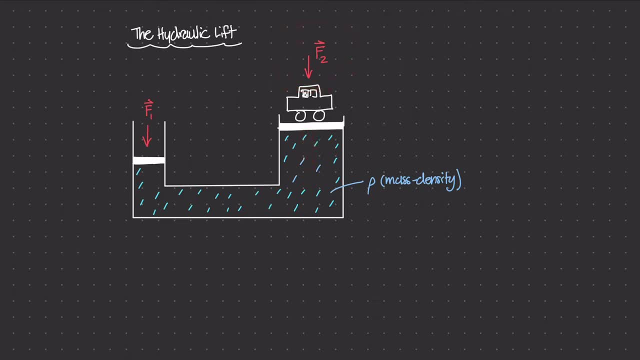 we can use to counteract F2.. We're also going to get into the term which is force multiplication factor. Now, this term is pretty important in hydraulic systems, especially hydraulic lifts, and the kind of very basic definition of this multiplication factor is that we can use two. 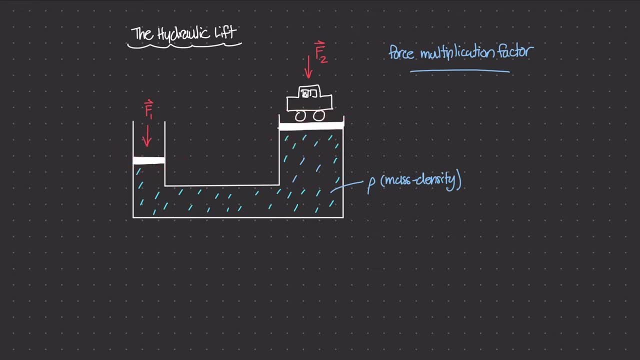 different areas of these pistons and the ratio between these areas is what we call the force multiplication factor. So what it does is that ratio between these two areas will amplify force 1 and the ratio between these two areas will amplify force 1.. So if we increase pressure at 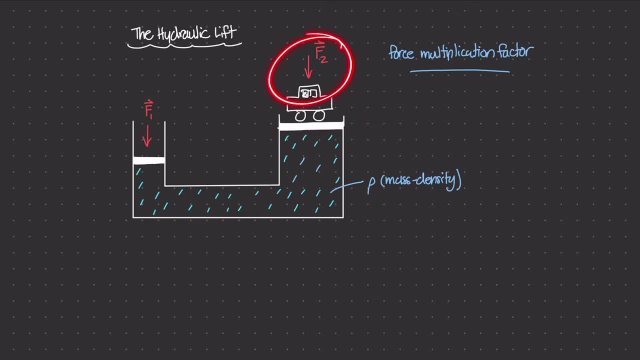 one point in the system, then that pressure is going to be applied against this big area for piston 2.. Now we're going to do this on the second piston to counteract F2. We'll get into that in a little bit, but as I said before, when we applied F1 to this hydraulic system on piston 1, that produced some 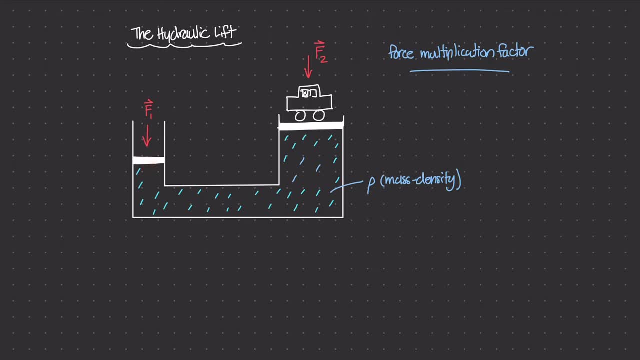 sort of a pressure right here Now, if I go ahead and I draw a line right where that pressure was induced by force 1.. So I'm talking about this line here. Well, what do we know about systems or fluids in this hydraulic system? Well, the first thing we know about is that the pressure is going to be. 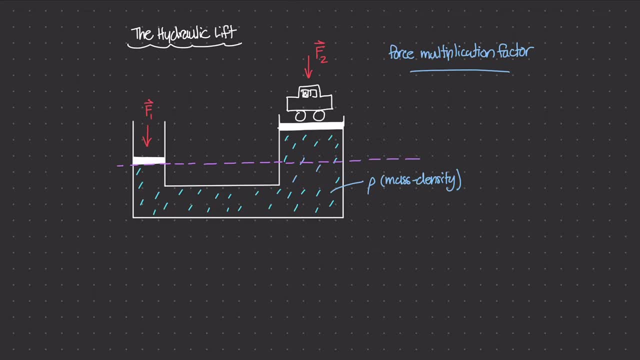 in height of static equilibrium. We know that if they're in compressible, which is the mass density's constant, then the pressure along this line is going to be the same for all points in that liquid along that line. Now you can see that piston 2, the piston on the right side is some. 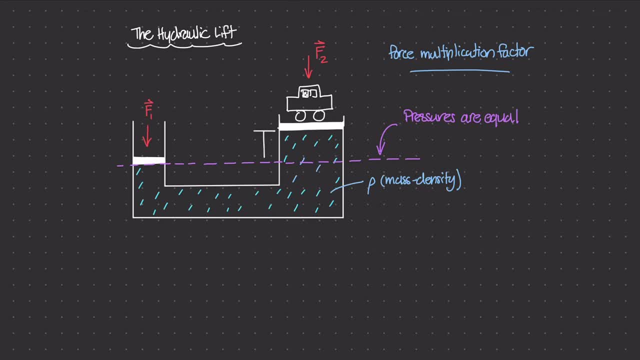 height above that line that we drew. So I'm going to call this line H. So this is just a height of H. Now this entire system is in static equilibrium, so we've applied some sort of force 1 to piston 1,. 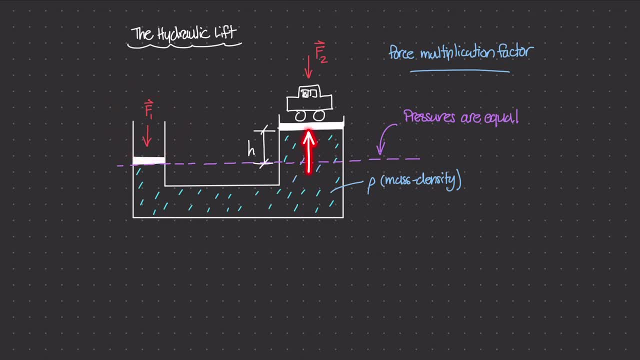 and that's resulting in some sort of resultant force here on the bottom side of piston 2, which is counteracting F2. So the car is not moving up or down, but we've applied some sort of force that's keeping the car on piston 2 from going up and down. Now how can we figure out what? 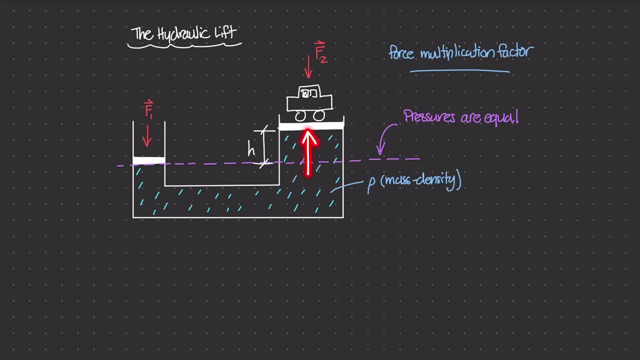 this counteracting force is. Well, we're going to have to look at some sort of force that's on the bottom of piston 2, or, in other words, the force required to balance out F2, based off of what we know about hydraulic systems, fluids in hydrostatic equilibrium and just the concept of pressures. 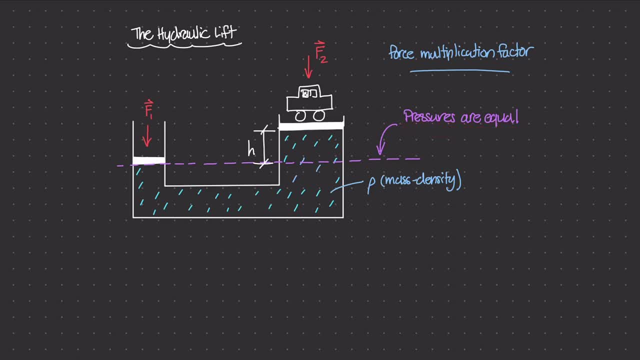 along horizontal lines. Well, what if we did this? What if we figured out a way to get F2 in terms of the areas of the piston 2?? Well, we're going to have to look at some sort of force that's going to apply to the pistons as well as the force 1 being applied on piston 1.. And if we do that? 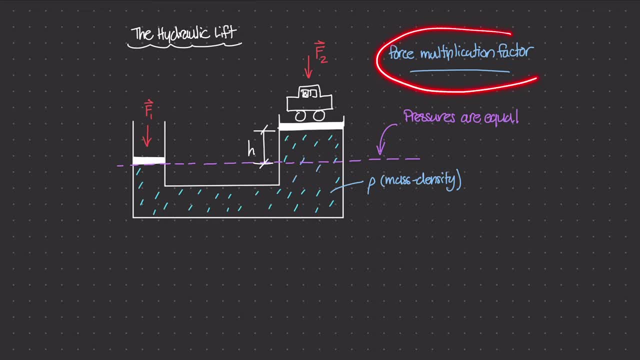 that's going to actually explain what this force multiplication factor is in hydraulic systems. So why don't we go ahead and try to do that? So what I'm going to do is I'm going to label two points along this purple line: here And on piston 1,, right where we're applying F1, there's going to 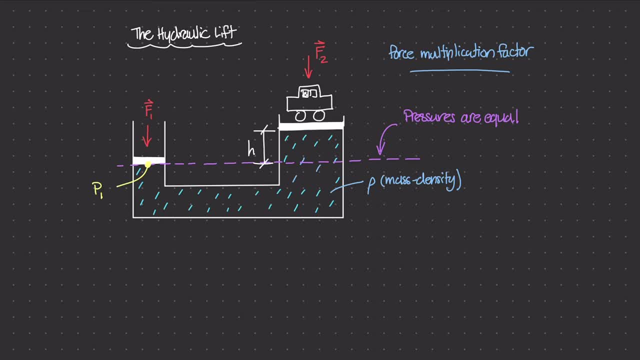 be a pressure induced at that point. right, And I'll just call that P1.. Now, along the same horizontal line over in piston 2, I'm going to draw another point and this is going to be P2.. Now, because I've drawn these two pressure points along that same line, I know that P1. 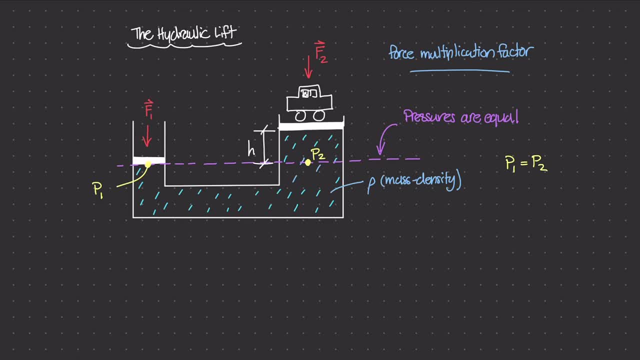 is going to equal P2.. But how can we use this concept to actually figure out what F2 is? Well, I think a good place to start is actually calculating what P1 and P2 are, based off of the forces being applied to the system. To start off here on P1: over on the left side, P1 is going to 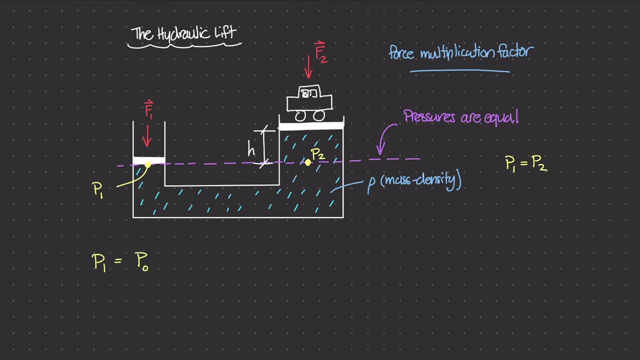 be equal to some sort of P0, so whatever P0 is being applied at the piston on the left, plus rho GD, plus the pressure caused by the piston on the left, So that's going to be P1 over on the piston 1.. So that's just going to be F1 over A1, and A1 is just the area of the piston. 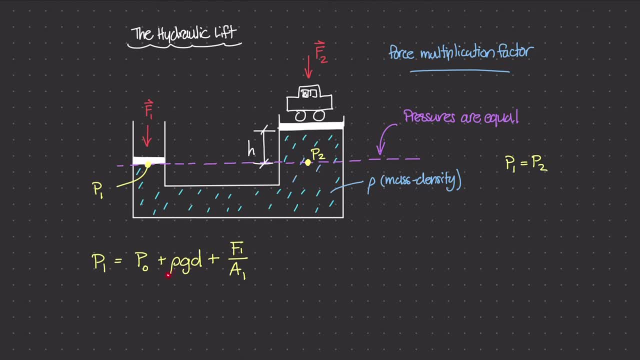 Now there's a couple things to note. This rho GD term is well. D is always the distance from P0 down to the point that we're studying, And since P1 and P0 are at the same point, our D is going to be equal to 0. So this term is actually going to go. 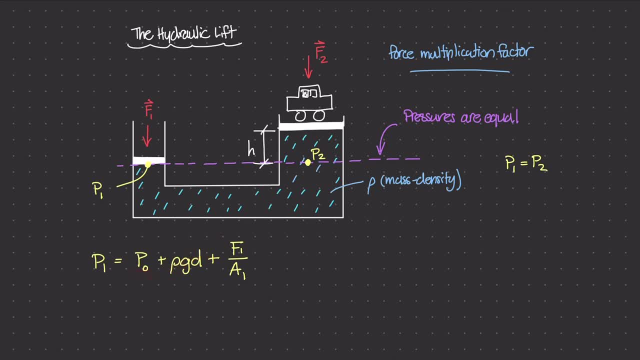 to 0.. So what we're really left with is just P0,, whatever external pressure is being applied to piston 1, plus the force over the area caused by this force right here. So I'll just go ahead and rewrite that It'll. 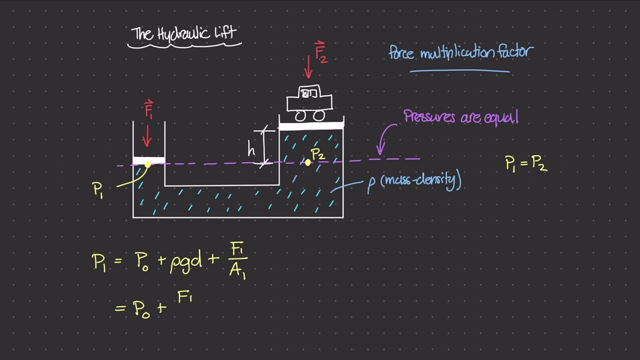 be P0 plus F1 over A1.. Well, what about pressure 2 here on the right side? So pressure 2 is going to be the same thing. It's going to have some sort of P0 being applied to the piston 2, plus rho GD. 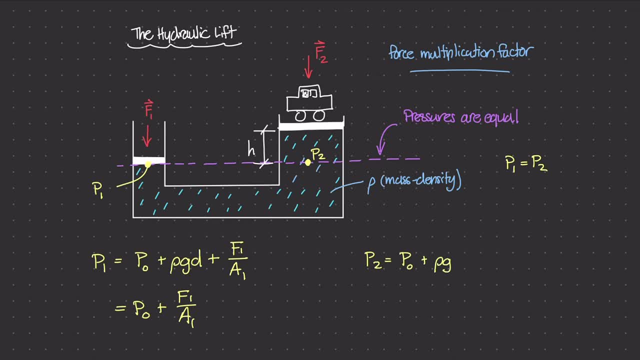 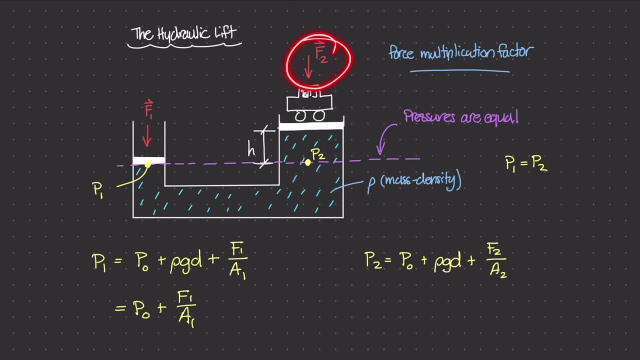 pressure being applied by this force right here. Now a couple things to note here. The first one is P0.. P0, again is just the, in this case just atmospheric pressure being applied to piston 2.. This rho GD term, remember it's. 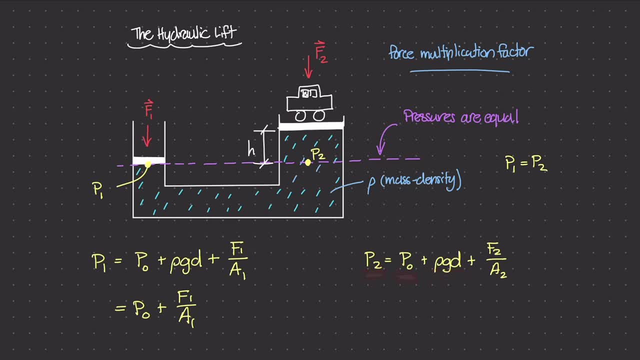 from P0 down to the point that we're studying. So P0 is being applied on into and the point that we're studying is here along the purple line, so that d, distance is actually this h value that I have marked. so really, this d is h. and then, finally, this last term, f2. 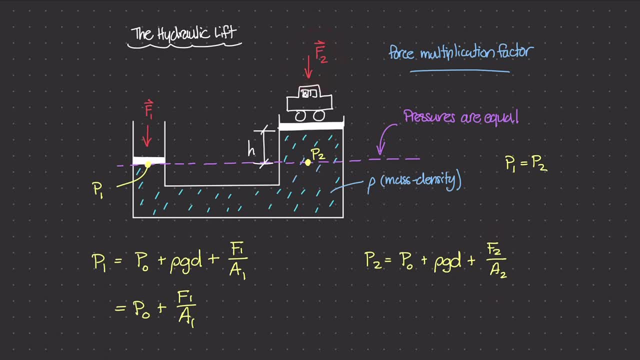 over a2. that's just the force of the car pushing down on the area of the piston. Now I did say that p1 and p2 are equal to one another. so I'm going to go ahead and set these two equations equal to each other and then we can actually solve for f2 in terms of rho. p naught a2, a1 and f1.. So I'm 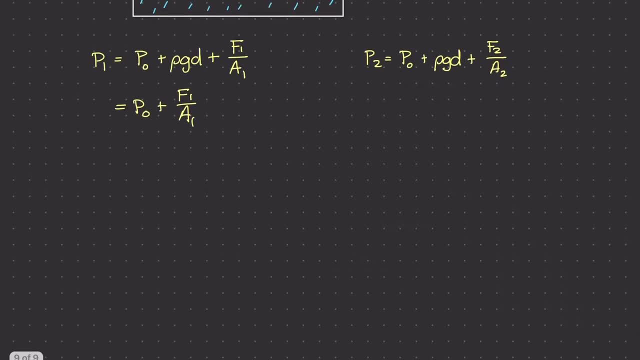 going to scroll down just a tiny bit and I'll say: p1 is equal to p2. so on the right side, p naught plus f1 over a1, this is equal to p naught plus rho, g, d and d was h right, the the height from. 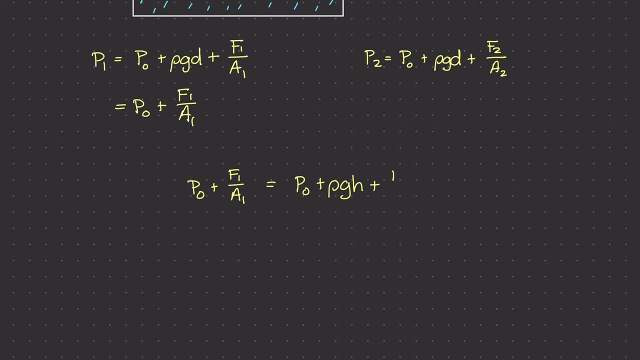 piston 2 down to p. Now you can actually see that p naught and p naught cancel out because they are constant. so we're left with f1 over a1 is equal to rho g, h plus f2 over a2.. Now, remember, we're trying to solve for f2, we're 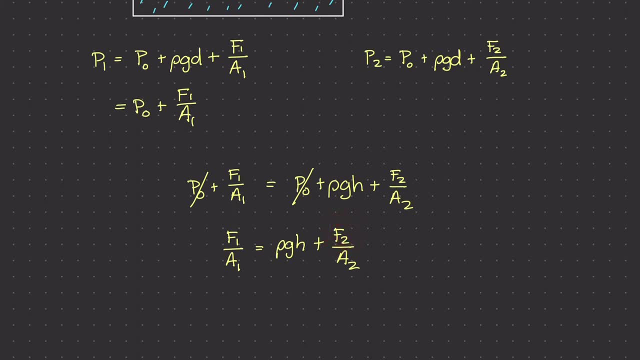 trying to figure out what that counteracting force is on piston 2 in terms of f1, a1 and a2.. So what I can do is I can subtract rho g h from both sides and we're left with f1 over a1 minus. 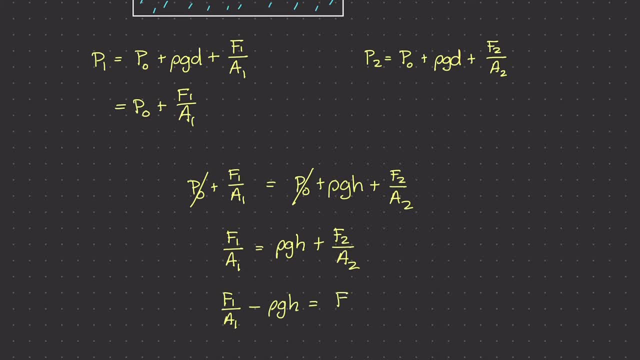 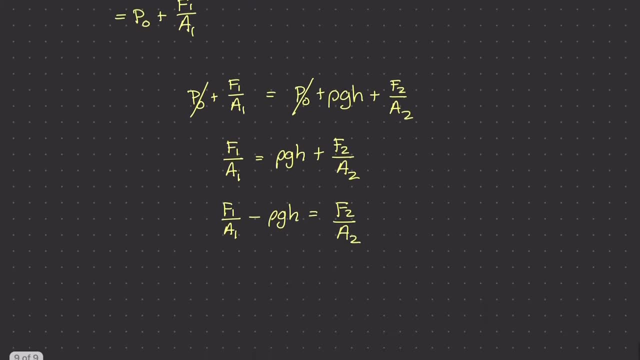 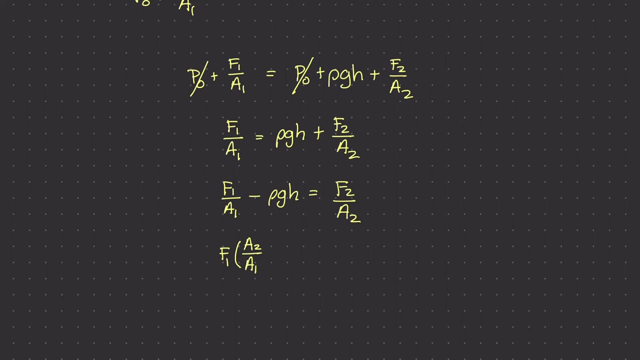 rho g h is equal to f2 over a2.. Now if we multiply both sides of the equation by a2, then we are left with f1, which is a2 over a1, minus rho g h times a2, and that is a2 over a1. 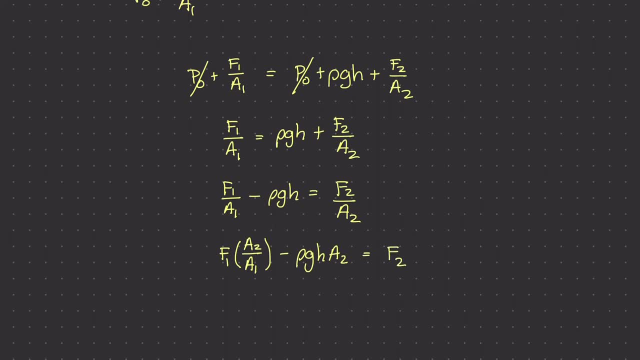 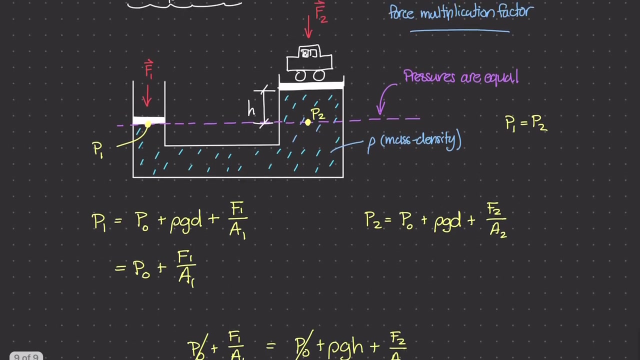 So this is equal to f2.. Okay, awesome. so we figured out what f2 was in terms of f1, a1, a2 and, of course, rho, g, h. So whenever we have hydraulic systems like this or a hydraulic lift that is of this type of a, 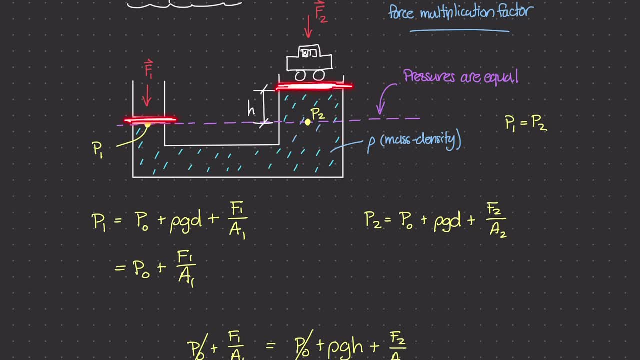 system where you have this larger piston on the right, this smaller piston on the left, you can apply a relatively small force and Pascal's principle is going to increase the pressure along all of these inner walls of this fluid and that will result in a larger force that gets to push piston 2 up. The force that's pushing piston 2 up is essentially 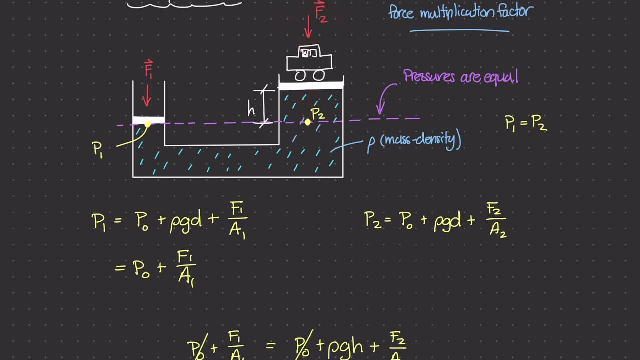 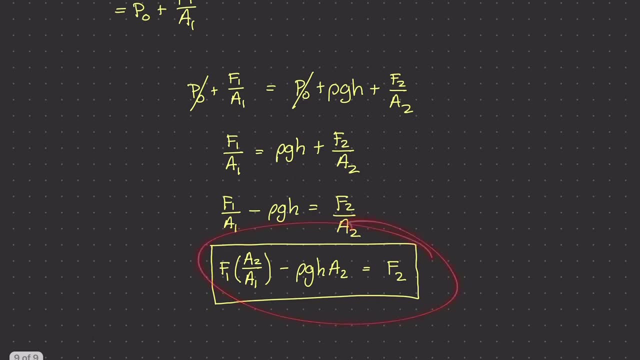 what f2 is. So in this case, just the force of the car pushing down on the piston- it's going to be counteracted by this f2 force that we found here. Now. that's pretty cool. so I want to draw your attention to one more scenario, and that's it'll help you figure out what f2 is. So let's start.